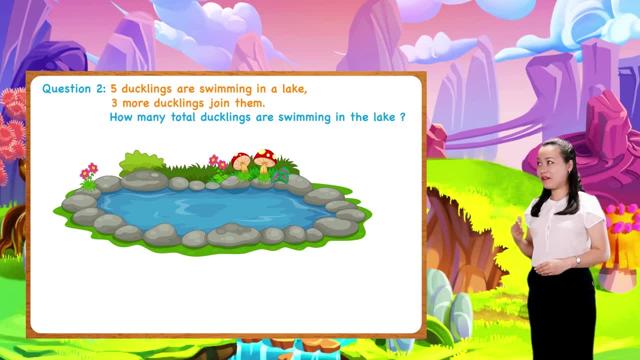 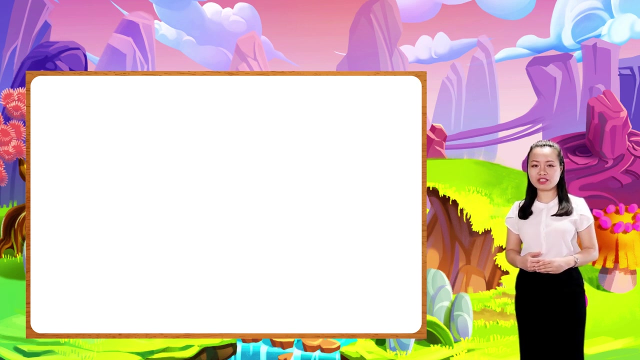 find the answer together. five ducklings are swimming in the lake. three more ducklings join them. we add five and three to find the total number of ducklings swimming in the lake. so five plus three equals eight. we conclude: total: eight ducklings are swimming in the lake. so we've solved some word problems. 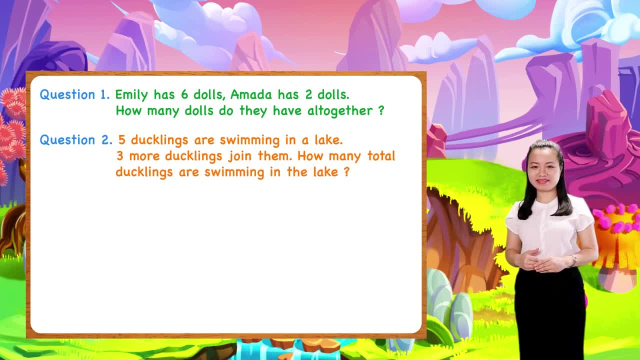 now we are going to solve the following problem. notice this: keywords altogether, they tell you to add. often you may see other keywords that also tell you to add, such as some in all both and combined. Now take a break for a while and then we'll move on to question 3.. 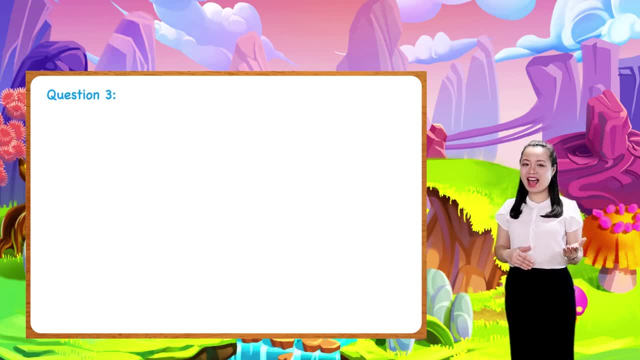 Question 3.. Andy has 4 toy cars. Pryan has some toy cars. They have 7 toy cars in all. How many toy cars does Pryan have? I'll give you some time to find the answer by yourself. Let's find the answer together. 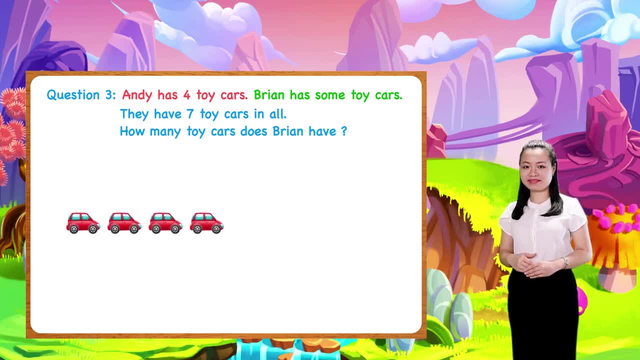 Andy has 4 toy cars, Pryan has some toy cars. They have 7 toy cars in all. We write in numerals. We say 4 plus something equals 7.. Recall the addition facts We learned in lesson 6..